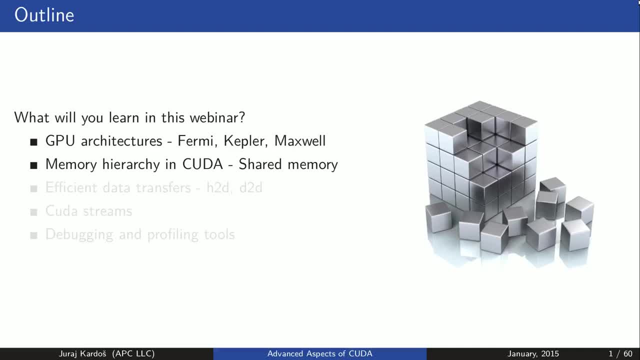 especially in memory intensive operations. We will focus on those aspects of memory hierarchy that are accessible by CUDA programming model. Therefore, you, as a programmer, can make an advantage of these features and further speed up your work. In this video, you will learn about charred memory, that is, low latency memory that can be used. 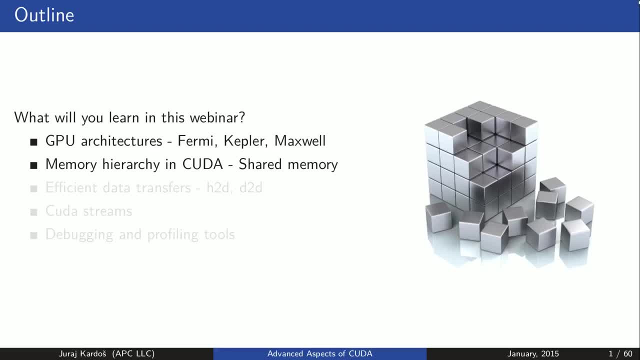 to cache your data and avoid expensive accesses to global memory. Efficient data transfers are closely related to memory system. Amount of transferred memory and the data communication path during the transfer have severe impact on the application performance. We will also introduce the concept of CUDA streams. that is necessary in order to 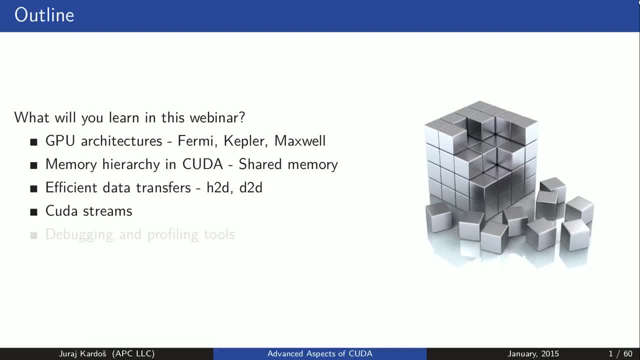 utilize simultaneous kernel launches within a single GPU or overlap communication with computation. And finally, we will introduce some debugging and profiling tools. During the project lifecycle, the code might grow huge or you may be dealing with code from a new project you are not familiar. 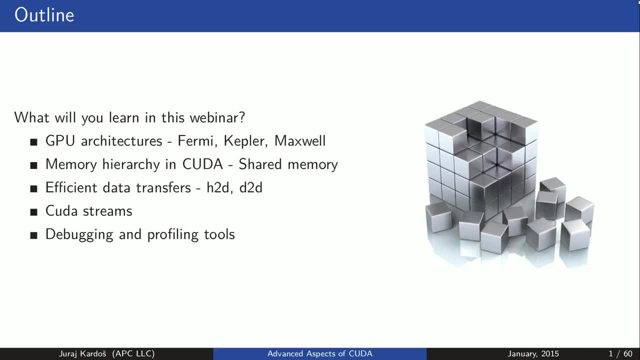 with. In such scenarios, it would be useful to have supporting tools that help you understand the code base, know where the bottlenecks are, and so on. We will introduce two different types of tools that are useful for the development of the project. 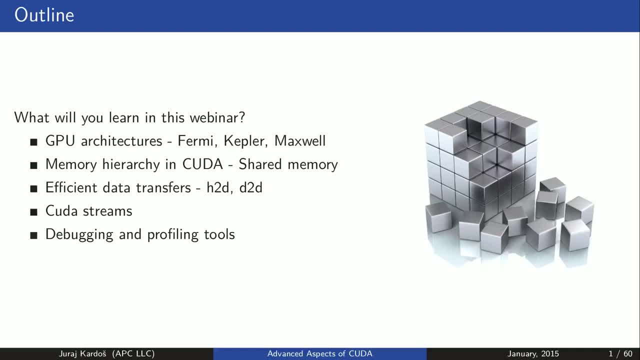 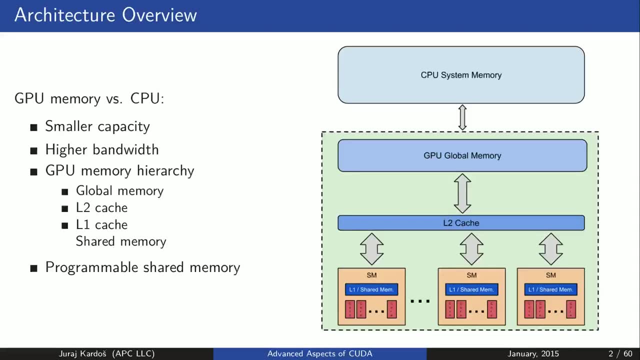 These tools are CUDA, GDB, CUDA MemCheck and NVIDIA Visual Profiling Tool. Let's have a look on architecture of CUDA capable GPUs. The choice of the execution unit's number, their latency and throughput is a central microarchitectural design task determining performance of the chip. 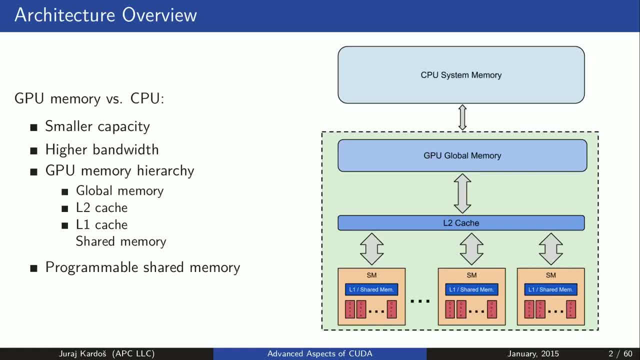 Understanding the basic architecture of whatever system you are programming for is necessary in order to create high performance applications. Most desktop systems consist of large amount of system memory connected to a single CPU which may have two or three levels of fully coherent cache. GPU memory hierarchy is in many ways similar. Typical system memory for CPU nowadays ranges: 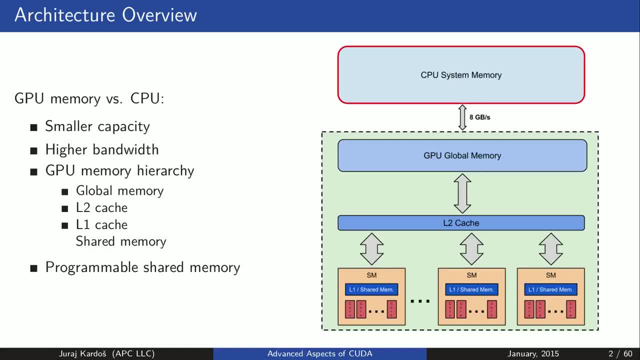 anywhere from 6 to 64 GB of system memory for the highest network stations. This system memory is connected to GPU via PCI Express with bandwidth of 8 GB per second. In case of PCI Express of second generation supported in Fermi 3rd generation, PCI Express doubles this bandwidth to almost 16 GB per second. 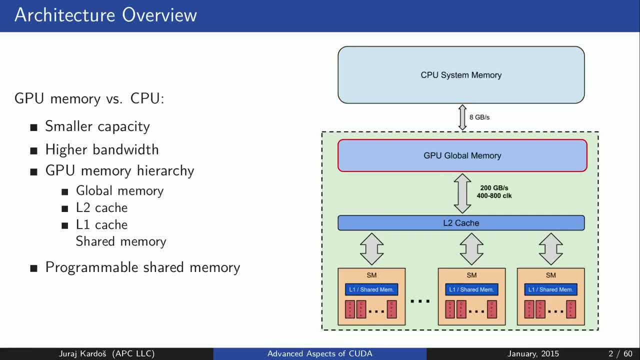 Note that the GPU has its own memory on board. That is, of course, global memory. Global memory size can be anywhere from 700 MB all the way up to 12 GB in case of Tesla K40, or 24 GB memory in Tesla K80 model. 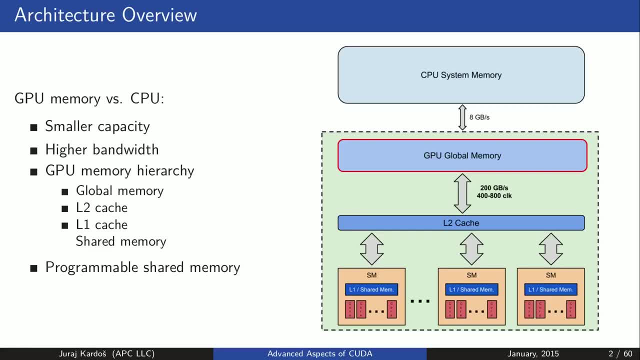 As you see, the trend is that GPUs don't have as much memory as CPUs, but the memory bandwidth for GPUs is usually substantially higher than that of even the highest end CPUs. Global memory bandwidth reaches 200 GB per second with latency of 4 to 800 clock cycles. 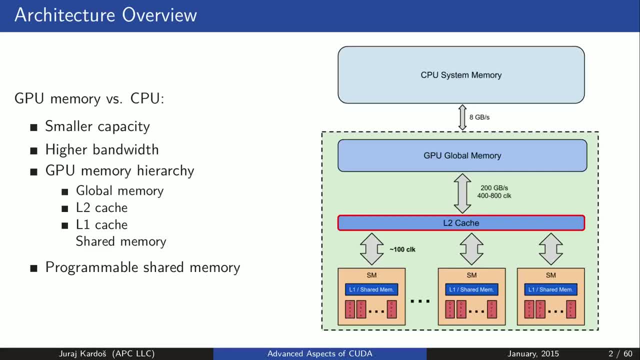 All modern CUDA capable cards, meaning Fermi architecture, and later have a fully coherent L2 cache. As with memory, the GPU's L2 cache is much smaller than a typical CPU's L2 or L3 cache, but has much higher bandwidth available. Latency of L2 cache is around 100 clock cycles. 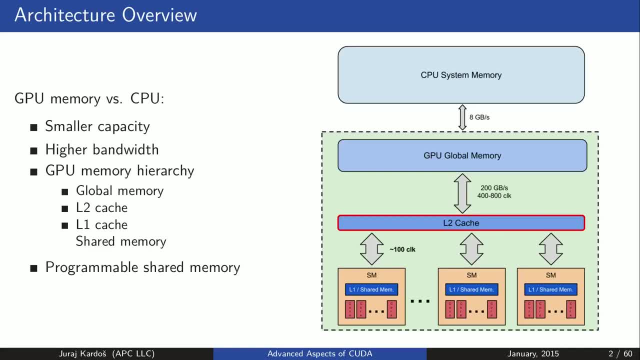 There is one L2 cache on chip, divided between streaming multiprocessors as needed. Finally, there is the L1 cache. High-end Nvidia graphic cards have multiple streaming multiprocessors and each is equipped with its own L1 cache. This memory provides low latency access, about 10 to 20 cycles. 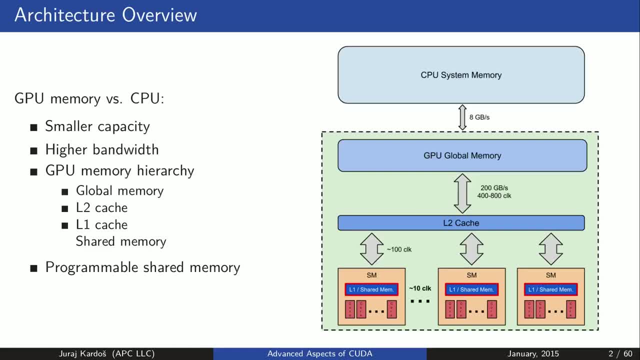 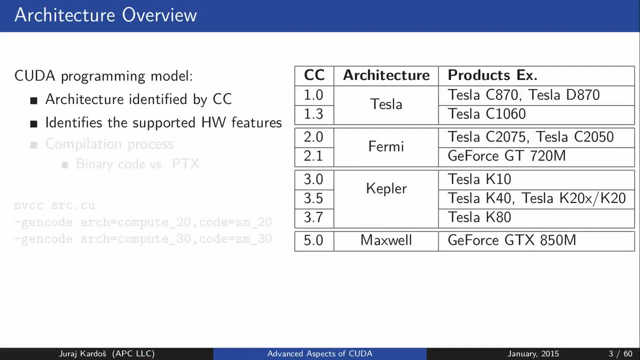 Other difference from CPU is that this fast L1 memory in GPUs can be programmable, or at least some portion of it, known as shared memory. We will talk about shared memory later in this video. In CUDA programming model, the specific hardware architecture is identified by compute capability. 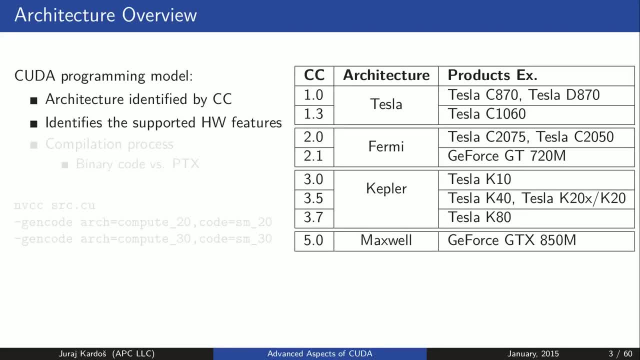 The compute capability of a device is represented by version number. This version number identifies the features supported by the GPU hardware and is used by application and runtime to determine which hardware features or instructions are available on the present GPU. The compute capability version consists of major and minor revision number. 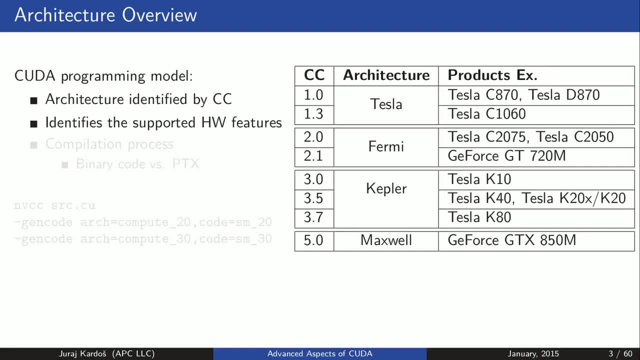 Devices with the same major revision number are of the same core architecture. The major revision number is 5 for devices based on the Maxwell architecture, 3 for Kepler architecture, 2 for Fermi architecture, 3 for Fermi architecture and, finally, 1 for devices based on the Tesla architecture. 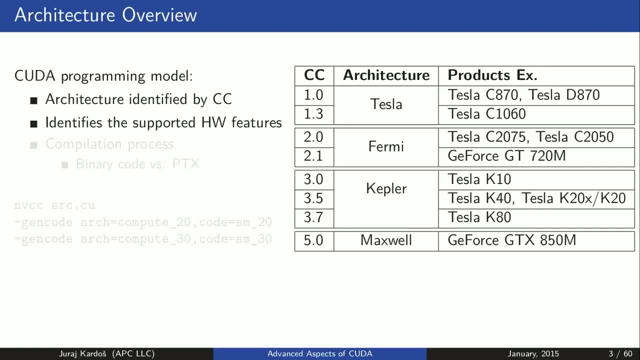 The minor revision number corresponds to an incremental improvements to the core architecture, possibly including new features. Compilation directives allows us to specify the target architecture. Source files compiled with NVCC compiler usually consists of mix of host code, that is, code that executes on the CPU, and device code. 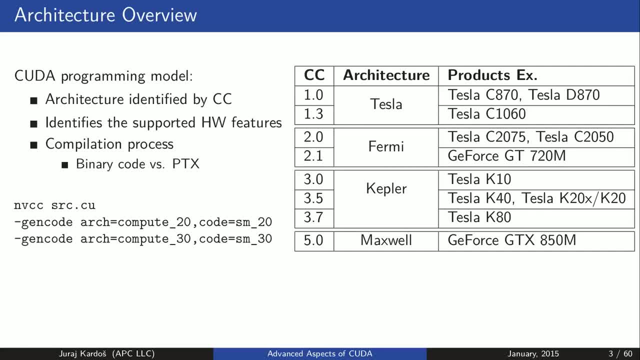 CUDA compilation works in a way that First CUDA device code is separated by CUDA frontend, replaced by a set of CUDA runtime function calls and passed to standard C C++ compiler. But what happens with the device code? It is of course compiled by NVCC. 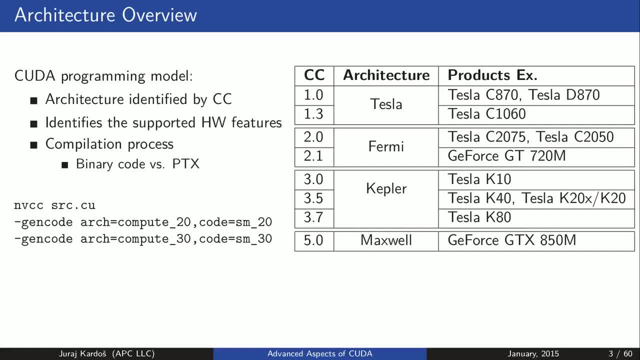 Depending on the value of the NVCC flags, this device code is translated by CUDA compilers into binary represented by a cubin object or into intermediate pseudo-assembly, PTX code. Binary code represented by a cubin object is architecture-specific. 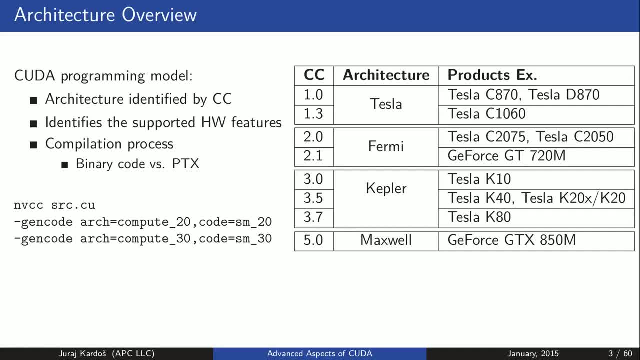 A cubin object is generated using the compiler option code that specifies the target architecture. For example, compiling with code XWALL equals SM. underscore 20 produces binary code for devices of compute capability 2.0. Binary compatibility is guaranteed from one minor revision to the next one, but not on. 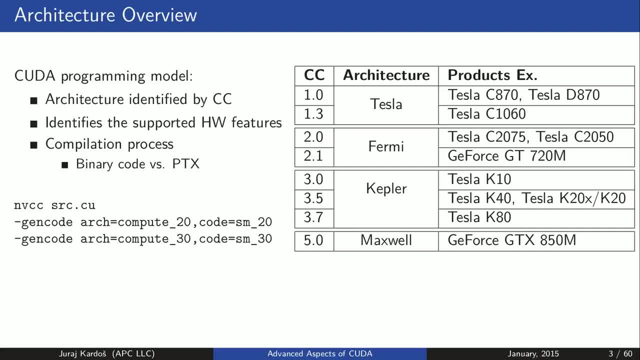 the previous minor revisions or across major revisions. In other words, a cubin object generated for compute capability 3.5 will execute only on devices with the same major revision number, that is, only on Kepler architecture, and with minor revision number that is equal or greater than specified for each revision. 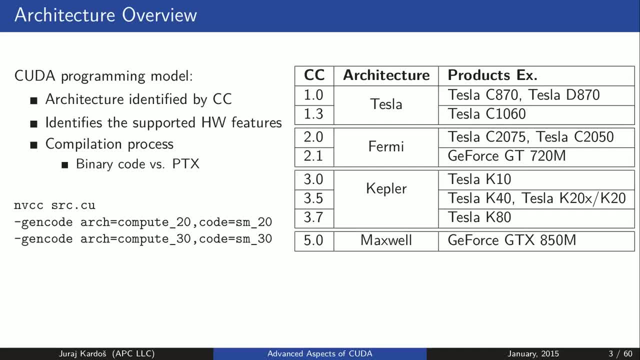 The virtual architecture specified by ARC option. in our case, for example, ARC equals compute underscore 20, determines what type of PTX code will be generated. PTX code loaded by an application at runtime is compiled to binary code by the device driver. 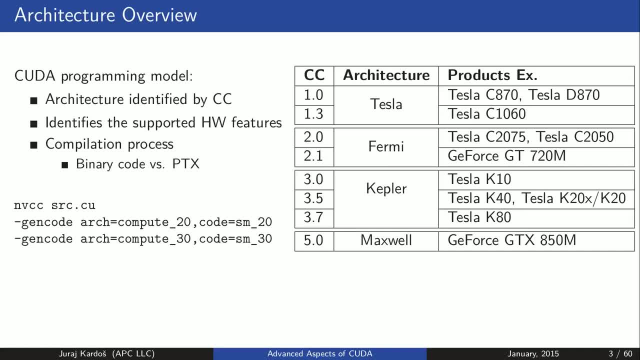 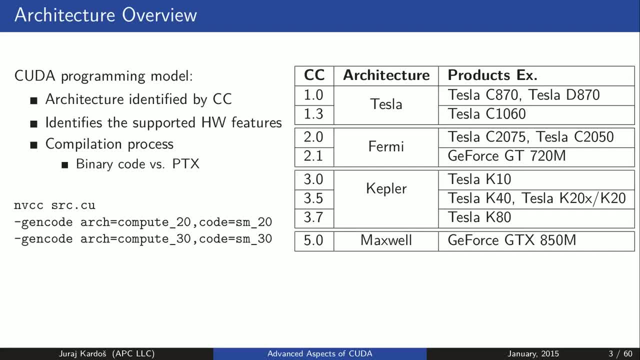 Specifying ARC option helps compiler to make presumptions about architectural features and generate more optimized PTX code than that default option that assumes compute capability 1.0.. As you can see in this example, you can specify multiple target architectures of your application. 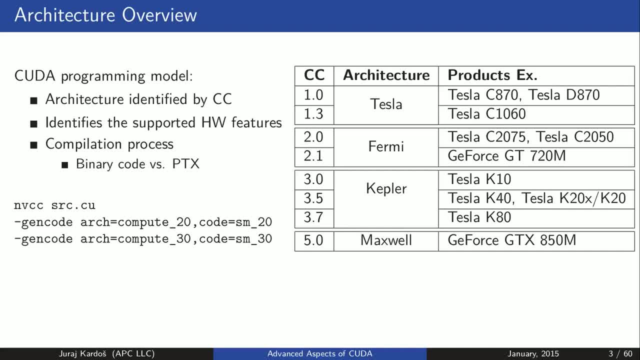 polarity trailer of your application multiplatform container. One advantage of including multiple virtual architectures, that is, multiple versions of PTX code, is that you have executable compatibility with a wider variety of target GPUs and your code will be better optimized for such target architectures. 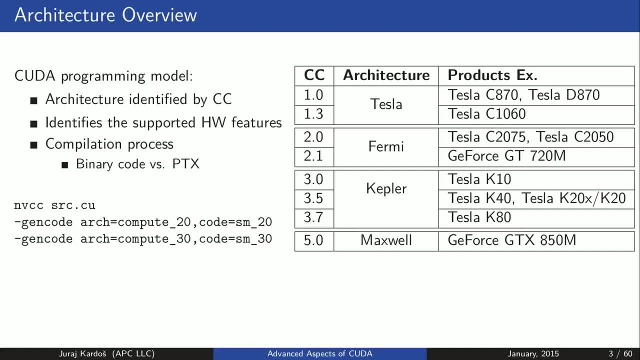 An advantage of including multiple binary GPU targets is that you can avoid just-in-time compilation step in case the GPU with specified compute capability is present. One possible disadvantage of specifying a lot of these options is code size bloat. Another possible disadvantage is compile time, which will be generally longer, as you specify. 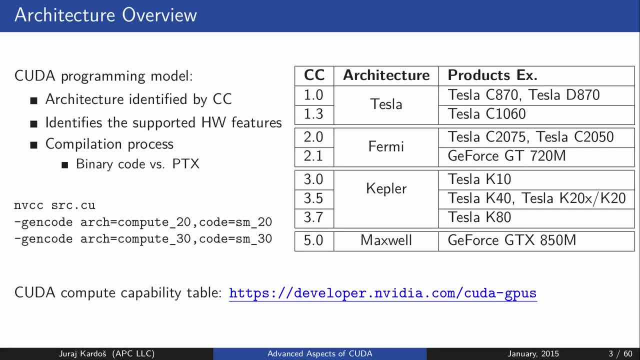 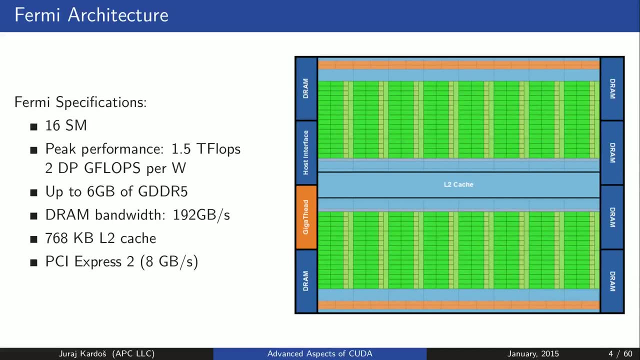 more options. You can find CUDA compute compatibility table under this link. it will give you information about architecture and compute capability of your Nvidia GPUs. We will start our architecture overview with Fermi. Fermi produced in 2010.. It has 3 billion transistors distributed within 16 streaming multiprocessors and control logic. 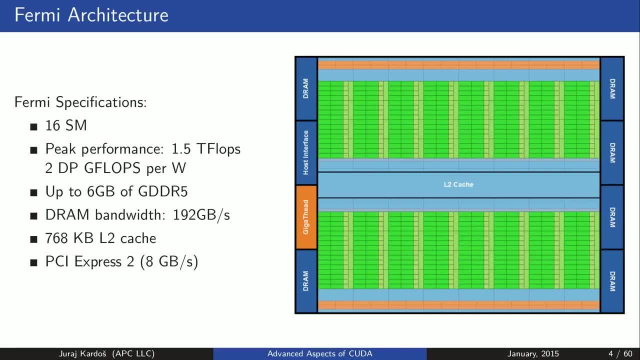 reaching peak performance in floating point of 1.5 teraflops. Fermi supports up to 6 GB of DRAM memory. thanks to the 64-bit addressing capability, DRAM bandwidth reaches 192 GB per second, and there is also an L2 cache on chip with capacity. 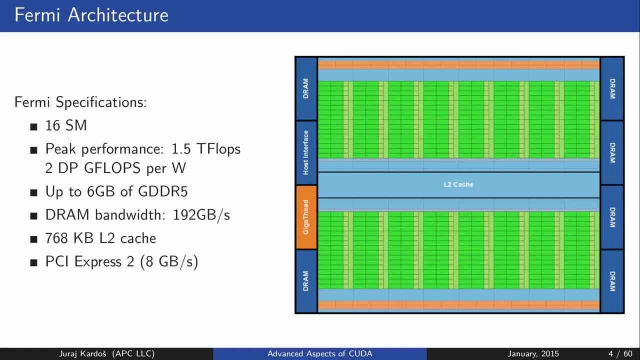 of 768 KB. Other subsystems on chip are: 1. Host interface, GigaThread, global scheduler and DRAM ports that connect to global memory. Host interface connects GPU to host via PCIe of 2nd generation. This transfer reaches peak performance rate of 8 GB per second. 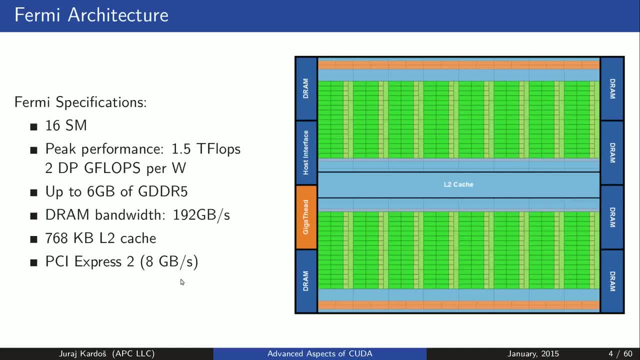 Notice the disproportion of the link between the global memory and host interconnect. You should adjust frequency of memory transfers according to this hierarchy. That is in ideal case. you minimize host disconnection. In other case, you minimize host device transfers and rather store intermediate data in global. 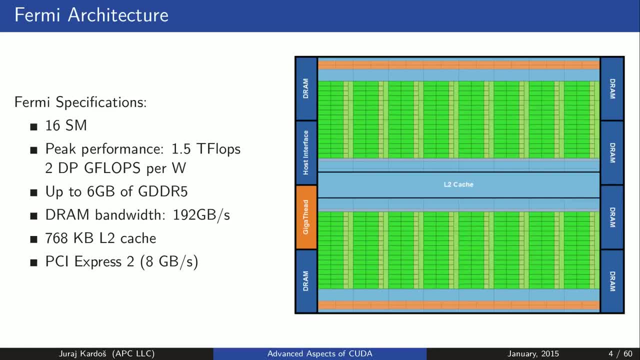 memory when you can access it more often as needed by an algorithm. However, global memory is also not appropriate for memory intensive operations. In such cases, you should use low latency and high bandwidth shared memory that we will discuss later. GigaThread global scheduler distributes thread blocks to streaming multiprocessors and its 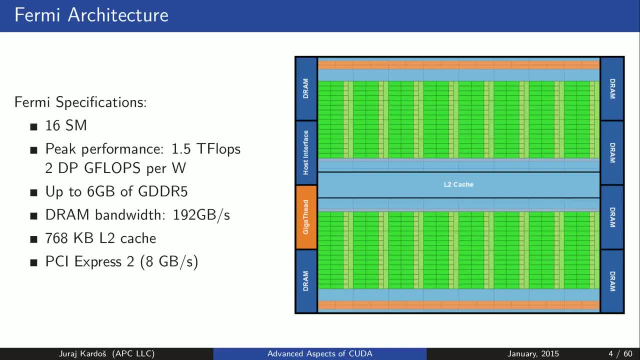 thread schedulers. It manages the context switches between threads during execution. As you know, in CUDA programming model the thread block is an abstraction of streaming multiprocessor and other abstractions in CUDA are Grid of blocks, that corresponds to GPU and thread that corresponds to a single CUDA core. 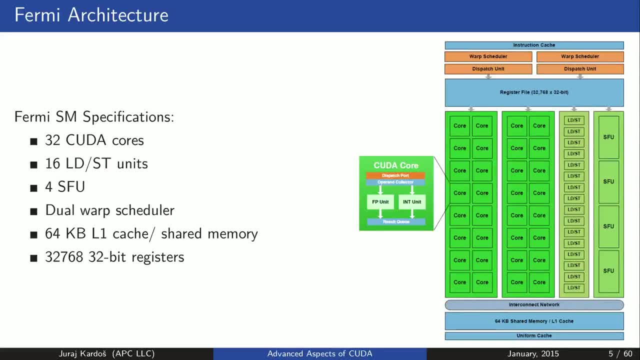 Let's have a closer look on the streaming multiprocessor. Each streaming multiprocessor in Fermi features 32 single precision CUDA cores And each core consists of integer and floating point unit. Floating point unit implements the IEEE floating point standard, also providing the fuse multiply. 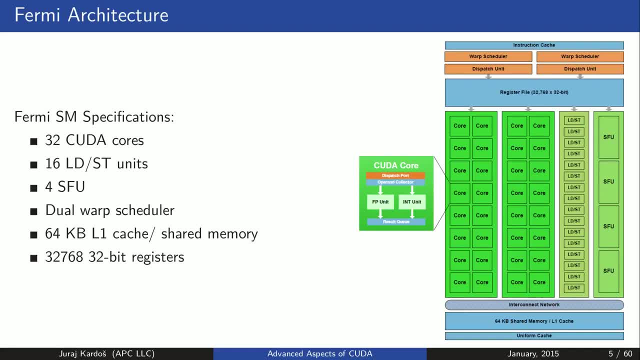 of the instruction. Load store units allow source and destination addresses to be calculated for 16 threads per clock. Special function units execute transcendental instructions such as sine cosine and square root. When it comes to workload scheduling, The GigaThread global engine schedules thread blocks to various streaming multiprocessors. 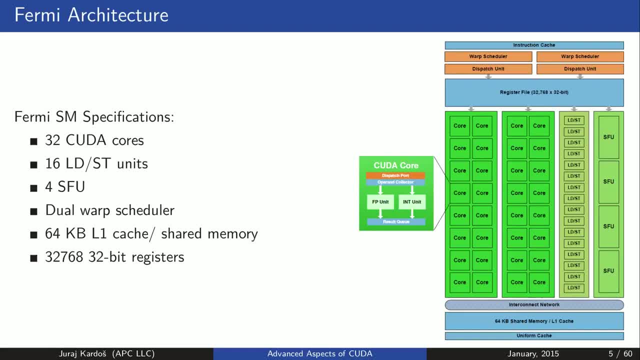 Further workload distribution is done on individual streaming multiprocessor level. Each streaming multiprocessor contains dual warp scheduler, where each warp scheduler distributes warps of 32 threads to its execution units. Execution unit is one of the four columns, two 16-core execution units, one unit of 16. 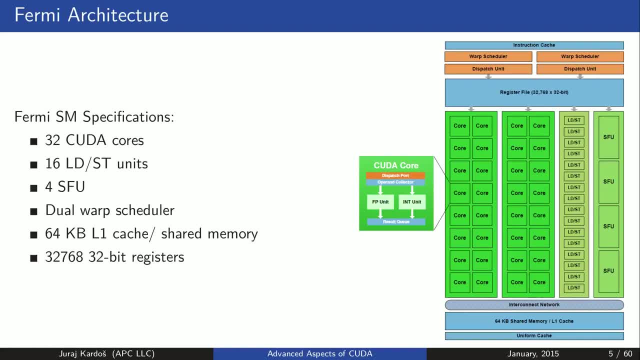 load store blocks or execution unit of four special function units. Each streaming multiprocessor features two warp schedulers and two instruction dispatch units, allowing two warps to be issued and executed concurrently. Each streaming multiprocessor contains on-chip memory that can be used either to cache data. 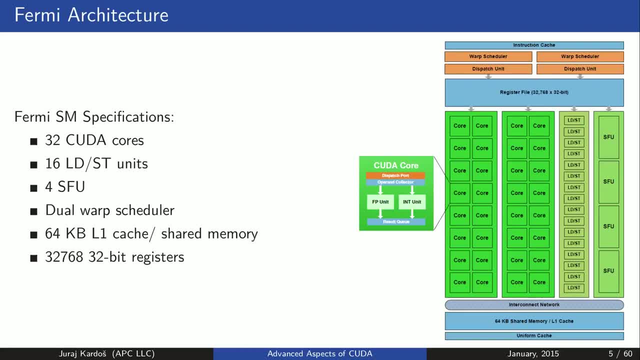 for individual threads or to share data among several threads. Shared memory: Shared memory enables multiple threads. Shared memory enables multiple threads. Shared memory allows multiple threads. Shared memory enables multiple threads within the same thread block to cooperate, enables extensive reuse of on-chip data and greatly reduces off-chip traffic. 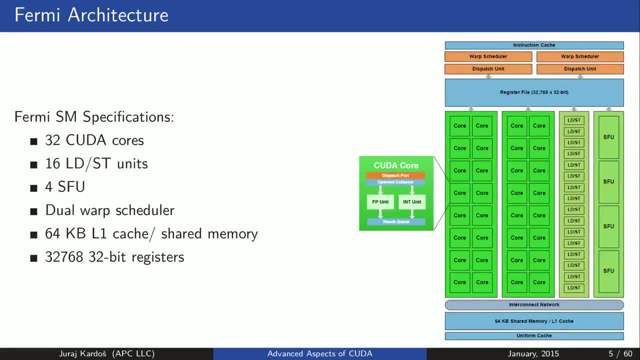 There is also a set of 32 thousand registers. In ideal case, there should be multiple blocks executing on the streaming multiprocessor at the same time. Also, each block has its own set of registers. This can happen only if the total number of requested registers can be satisfied for each. 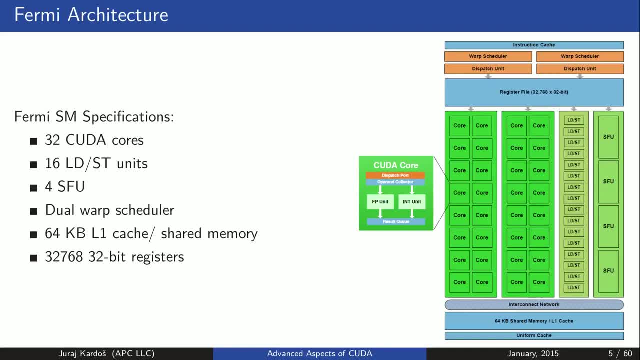 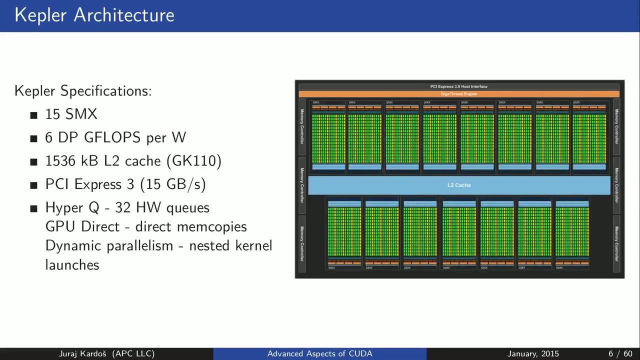 block. If multiple blocks do not fit to streaming multiprocessor, they request more registers than available. then just as many blocks run so that all can be granted. requested number of registers. If single block requests more than 32,000 registers, out-of-resources error will be returned. Kepler architecture produced in. 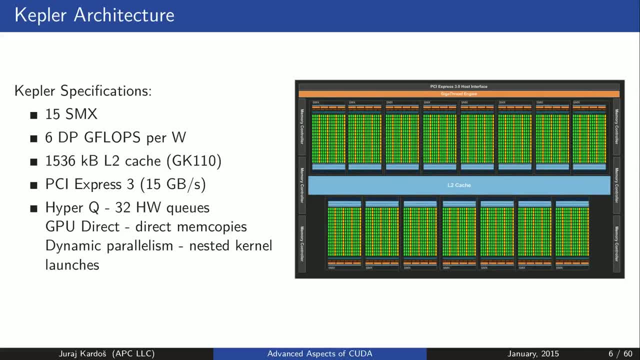 2012 consists of 7 billion transistors distributed within 15 streaming multiprocessors. While the goal of the previous architecture was focused on increasing pure compute performance, the Kepler architecture focuses also on the energy efficiency and programmability Today the primary constraint on processor. 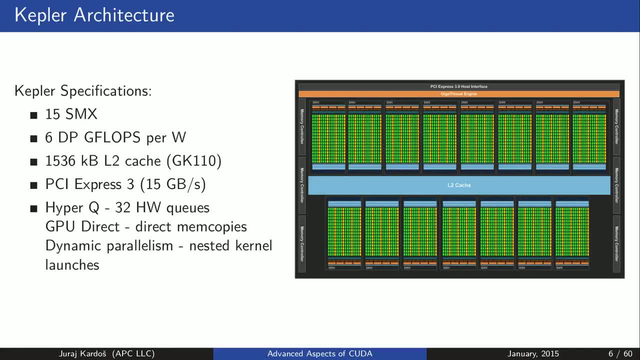 performance is the power consumption budget. Having a more efficient process enables us to add more processing cores, thus increasing performance. Kepler achieves six double precision gigaflops per watt, while Fermi achieves only two in high-end Nvidia GPUs. Global memory characteristics remain the same as in the previous architecture, The Kepler GK110. 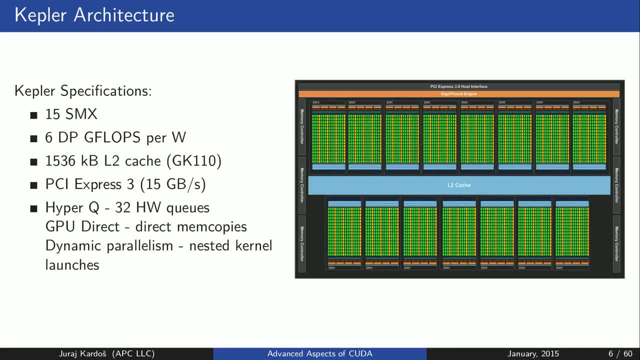 GPU features one and a half megabyte of dedicated L2 cache memory. that doubles the amount of L2 cache available in the Fermi architecture. Kepler introduces new version of PCI Express that doubles the bandwidth of second generation used in Fermi. Kepler also introduces new technologies such as: 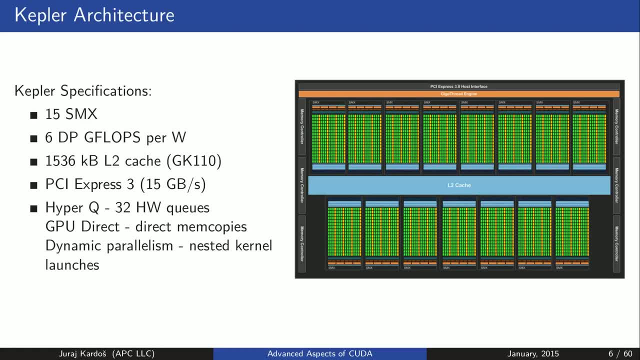 HyperCue, Dynamic Parallelism or GPU Direct. HyperCue increase number of hardware work queues from 1 to 32, which enables multiple CPU threads or processes to launch work on a single GPU simultaneously. Having a single work queue meant that Fermi could be under-occupied at times. 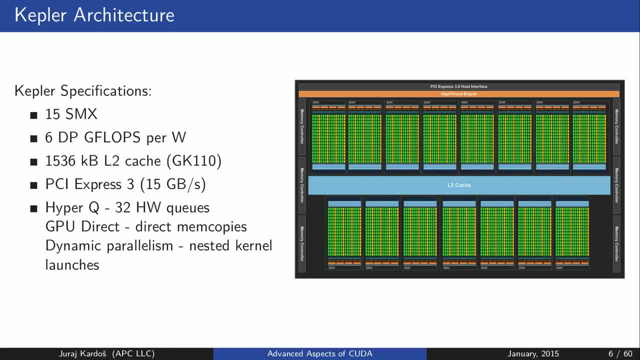 as there wasn't enough work to fill every streaming multiprocessor By having 32 work queues. Kepler can in many cases, achieve higher utilization by being able to put different task streams on what would be otherwise idle streaming multiprocessors. GPU Direct allows communication to directly exchange data. 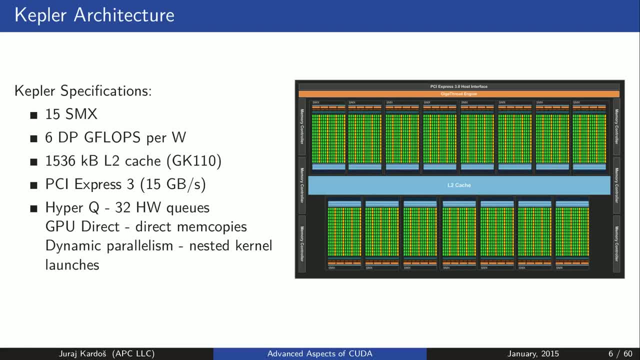 without needing to go to CPU system memory. The DMA feature in GPU Direct allows third-party devices such as SSDs or network card adapters to directly access memory on multiple GPUs within the same system, which significantly decreases the latency of MPI messages to or from GPU memory. Dynamic Parallelism allows threads to 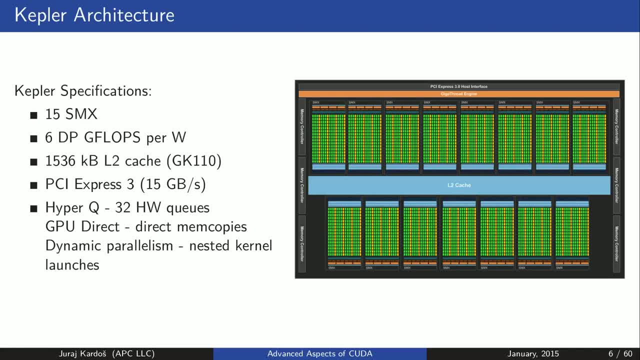 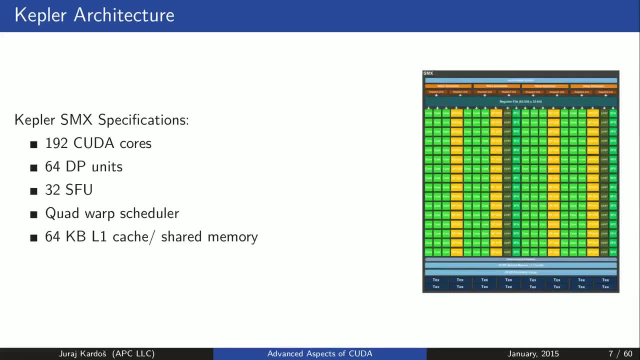 launch other kernels which can simplify programming your application. in some cases, The Kepler architecture employs a new streaming multiprocessor architecture called SMX. Kepler uses a new streaming multiprocessor architecture called SMX. to be used, Kepler reduces the amount of control logic and increase the number of CUDA cores. 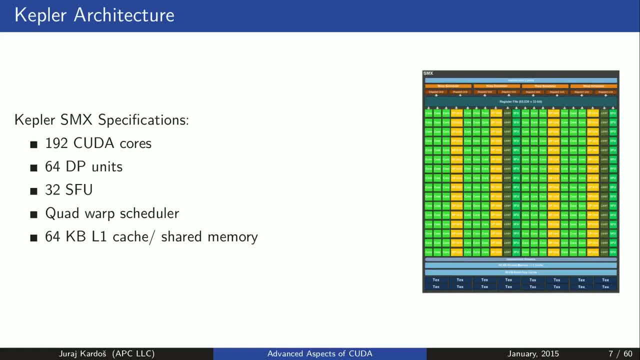 six times when compared to Fermi streaming multiprocessor. Because all the Kepler CUDA cores run at a lower clock speed than in Fermi, the GPU as a whole uses less power, even though it delivers more performance. Primary focus was put on energy efficiency, resulting in 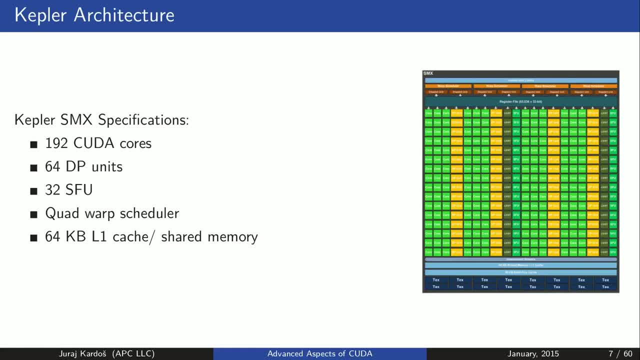 fact that two Kepler CUDA cores consumes 90% power of a single Fermi CUDA core. One of the design goals for Kepler was to significantly increase the GPU's delivered double precision performance, since double precision arithmetic is in heart of many high-performance computing applications. Kepler SMX also retains the 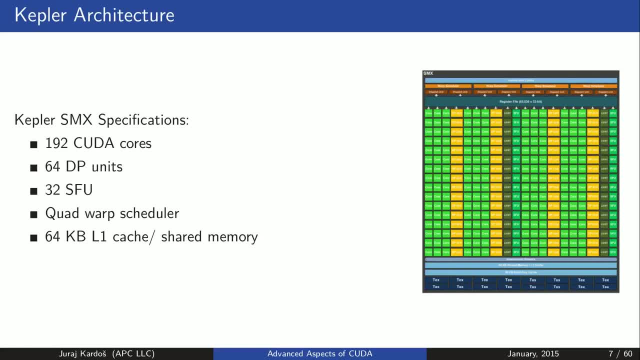 special function units for fast approximate of transcendental operations, providing eight times more special function units as the Fermi streaming multiprocessor. Each streaming multiprocessor features four- warp schedulers and eight instruction dispatch units, allowing four warps to be issued. 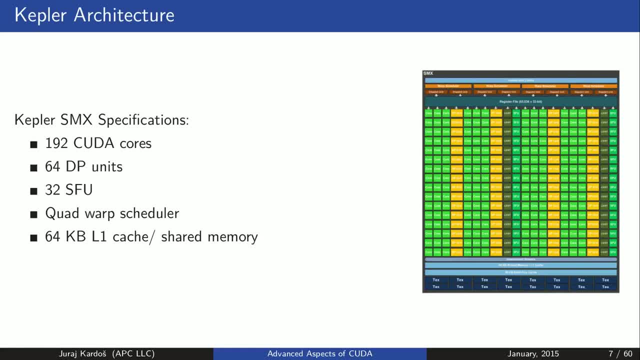 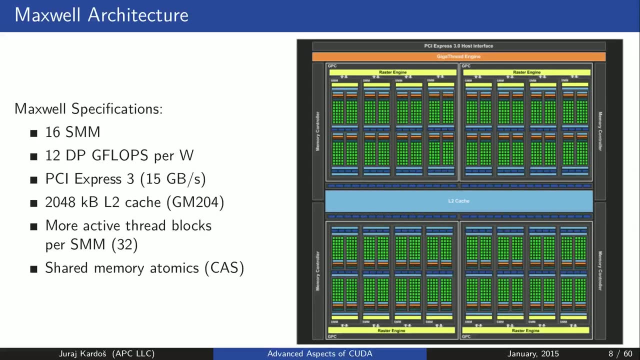 and executed concurrently. Kepler's squared-warp scheduler selects four warps and two independent instructions per warp can be dispatched each cycle. Compared to Fermi, only two warps could be issued and executed concurrently. Maxwell, released in 2014,, consists of 16 streaming. 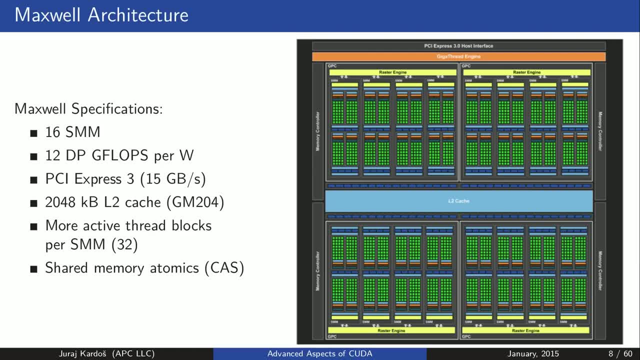 multiprocessors divided into four graphics processing clusters, reaching performance of 12 double-precision gigaflops per watt, making computation even more energy efficient than previous architectures. Host interconnectivity is implemented by PCI Express of third generation and L2 cache has grown to 2 MB. Having a larger cache, 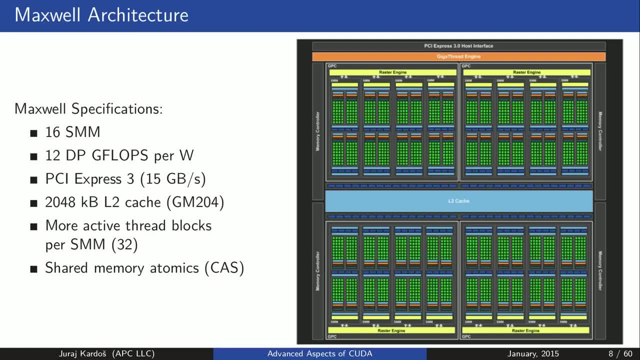 reduces the number of memory requests that have to be made to global memory. Maxwell increases the maximum active thread blocks per streaming multiprocessor from 16 to 42. This should help improve occupancy of kernels running on small thread blocks, such as 64 threads per block. 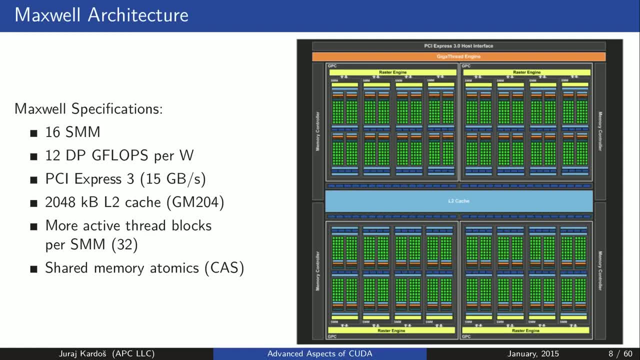 Kepler introduced large improvements to the performance of atomic operations to device memory, but shared memory atomics used a lock-update-unlock pattern that could be expensive in case of high conflicts for updates to particular locations in shared memory. Maxwell introduces native shared memory atomic operations for integers and uses the same. 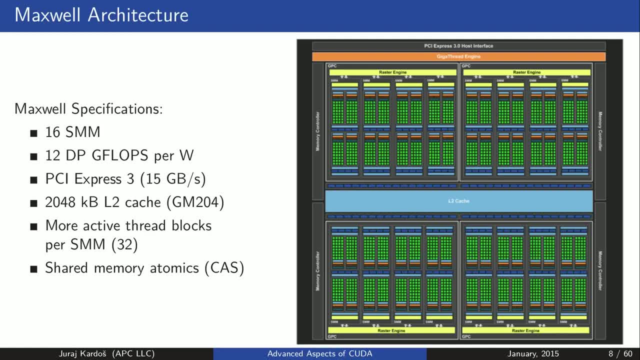 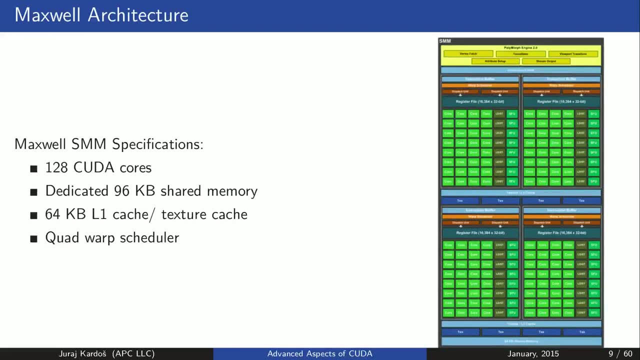 in the wide range of various tests. A native Compar Architecture web can be used to implement other atomic functions with reduced overhead compared to Fermi and Kepler methods. Maxwell has decreased number of CUDA cores in streaming multiprocessor to 128, which aligns with warp size. Having a core count being multiple over warp size makes it easier. 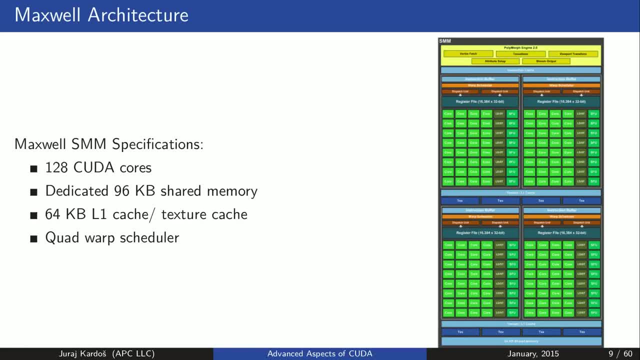 to utilize efficiently all CUDA cores. Savings are made also in terms of area and power that had to be spent to manage data transfer- to geç取于磾磾磾 fan store needed 것- and transfers in more complex organizations used by Kepler. 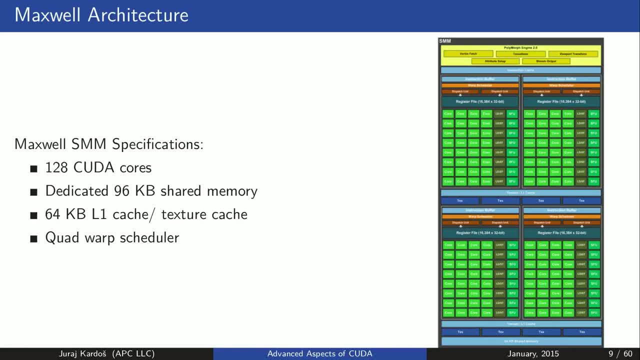 Maxwell further improves on Kepler by separating shared memory from L1 cache, providing a dedicated 96 KB of shared memory in each streaming multiprocessor. The per-thread block limit remains 48 KB also in Maxwell, but the increase in total available shared memory can lead to occupancy improvements. 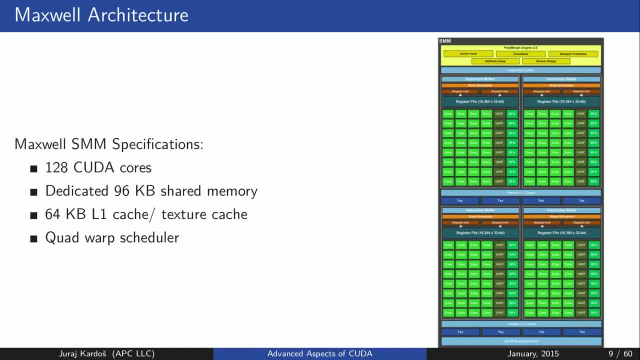 Shared memory is made possible in Maxwell by combining the functionality of the L1 and texture caches into a single unit. Each streaming multiprocessor contains four warp schedulers, and each warp scheduler is capable of dispatching two instructions per warp every clock cycle. 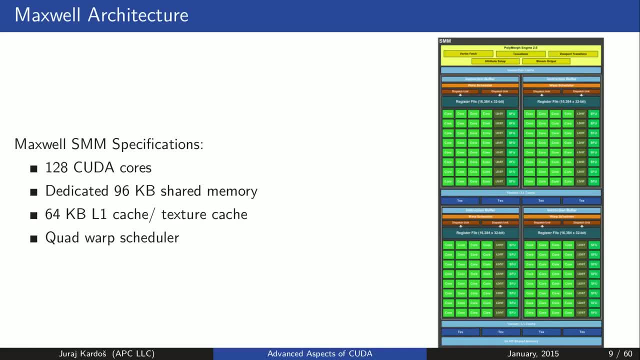 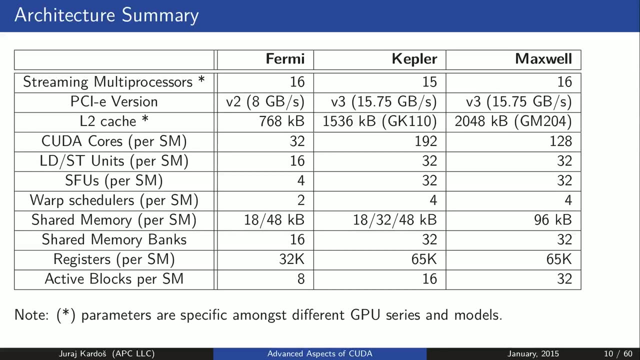 Compared to Kepler scheduling logic. a number of improvements in the scheduler were integrated to further reduce redundant recomputation of scheduling decisions. improving energy efficiency: We have seen how GPU architectures evolved, optimizing its performance and energy efficiency. Here you can see a short summary of the architectural features we have talked about in this section. 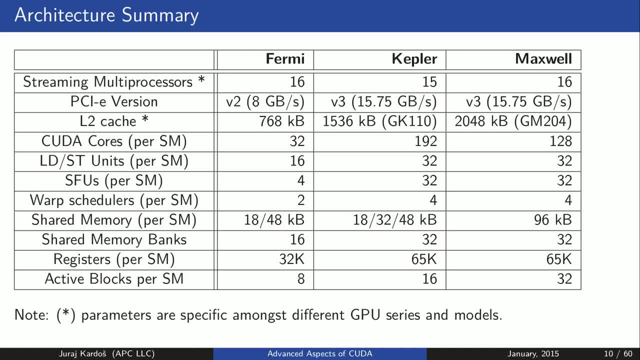 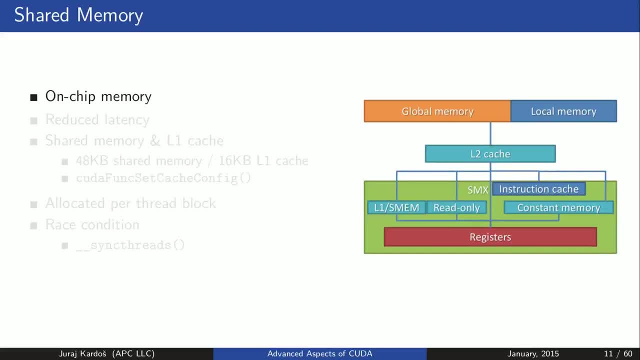 In the following part, we will have a closer look on shared memory and how to use it efficiently to improve performance of your applications. In this part, we will inspect properties and usage of shared memory. When you port applications to a shared network, you can use shared memory as an example. 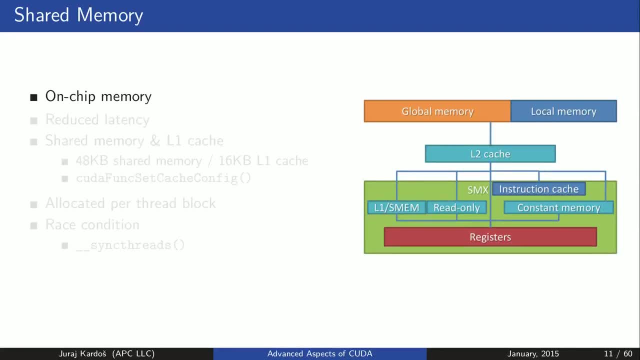 When you port applications to CUDA, you probably expect a massive speedup compared to a serial CPU code. Provided that you adhere to good CUDA programming practices, such as coalescing memory accesses or avoiding code divergence, and you still don't reach good speedup, you probably want 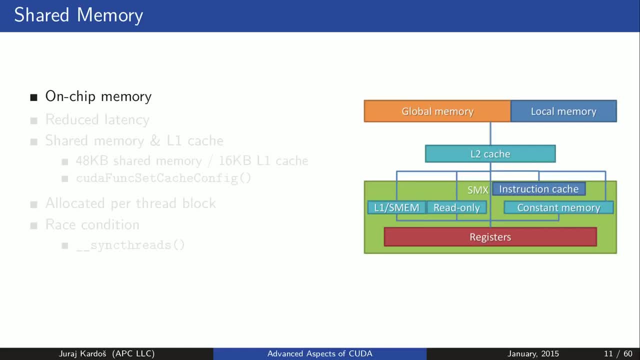 to inspect memory access patterns of your application. We have seen that memory transfer between host and device is done at 8 or 16 GB. in best case, We will see that PCI Express can be shared among multiple users or peripheral devices. therefore, the bandwidth can be even more reduced. 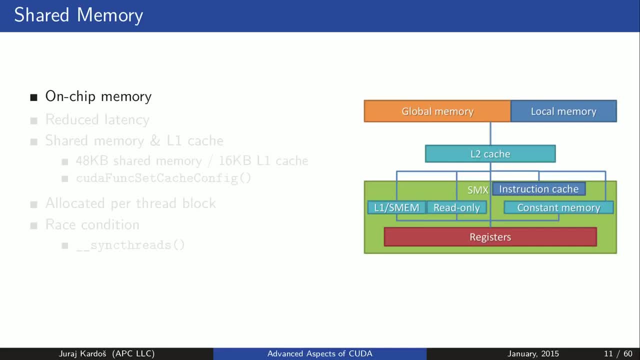 Memory access to global memory has bandwidth reaching 200 GB per second, while on-chip shared memory has bandwidth 1,600 GB per second and much lower latency Because it is on-chip, shared memory is much faster than local and global memory. In fact. 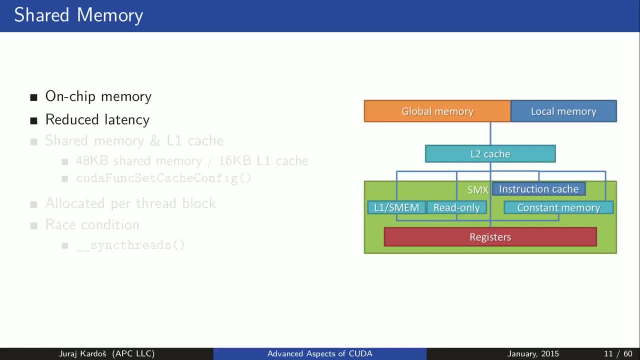 In fact, shared memory latency is roughly 100 times lower than uncached global memory latency, provided that there are no bank conflicts between the threads, which we will examine later in this section. On Fermi and Kepler devices, each multiprocessor has 64 KB of on-chip memory that can be partitioned. 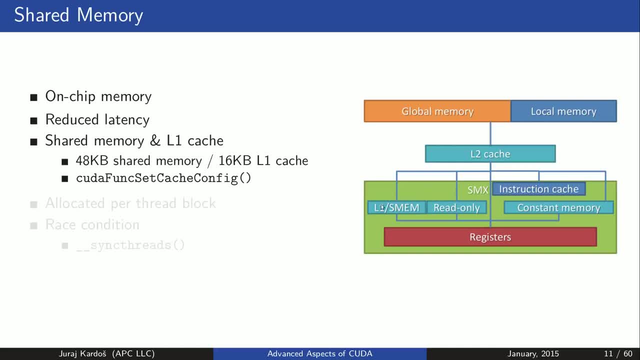 between L1 cache and shared memory. We are talking about this part of memory hierarchy, with CUDA cores being somewhere here. For devices of compute capability 2, there are two settings: 48 KB shared memory and 16 KB of L1 cache, and the other way around. 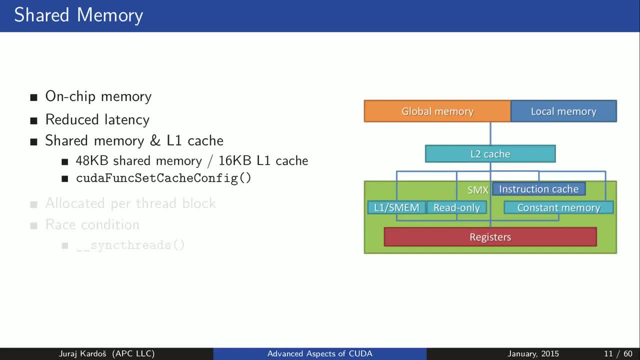 Devices of compute capability 3 and later allow the third setting of equal distribution of 32 KB shared memory and 32 KB of L1 cache. By default, the 48 KB shared memory setting is used. This can be configured during runtime using API function. 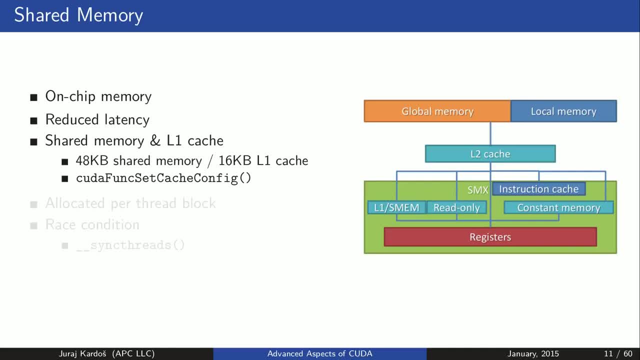 As we have seen in Maxwell architecture, shared memory is separated from L1 cache, providing a dedicated 64 KB of shared memory in each streaming multiprocessor. Shared memory is allocated per thread block, meaning that all threads in the same block have access to the same shared memory. 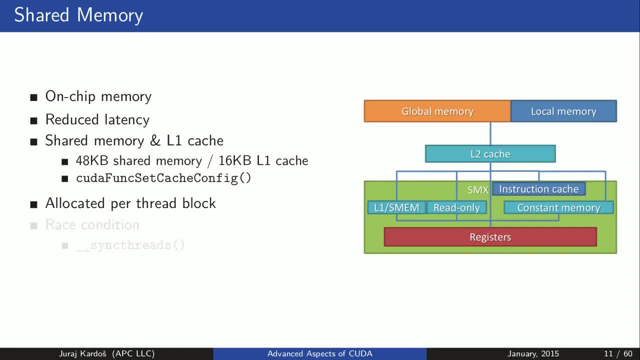 Threads can access data in shared memory loaded from global memory by other threads within the same thread block. When sharing data between threads, we need to be careful to avoid race conditions. While threads in a block run logically in parallel, not all threads can execute physically. 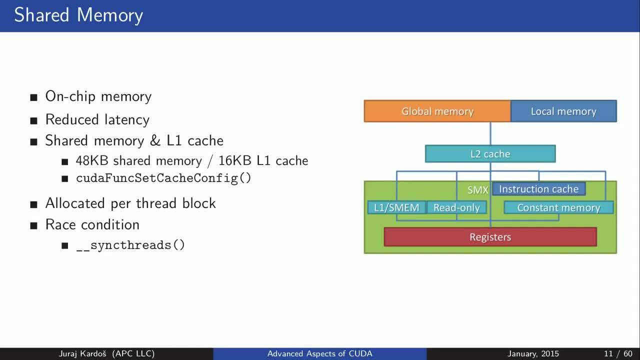 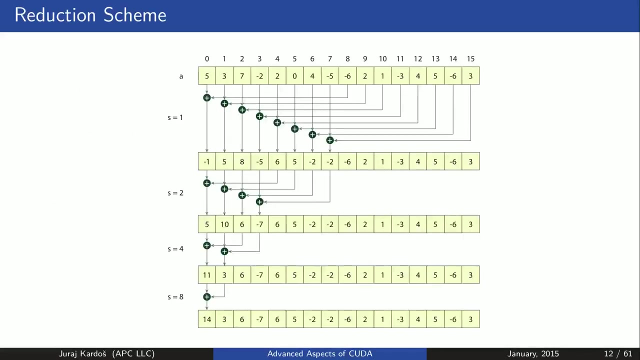 at the same time, To ensure correct results when parallel threads cooperate, we must synchronize the threads. CUDA provides a simple barrier synchronization primitive. A thread execution can only proceed this barrier after all threads in its block have reached this point. This is the general scheme of reduction we will perform. 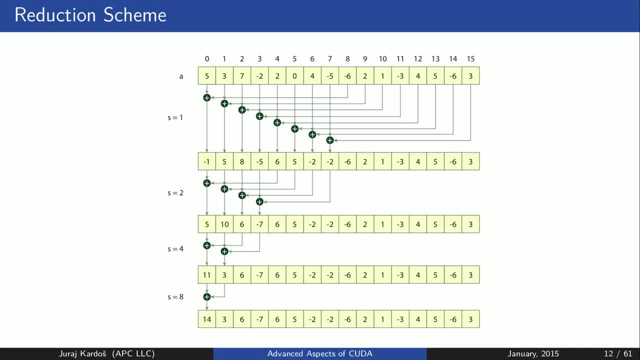 We have an array A that contains integers. we want to reduce using the plus operator, That is, we want to compute some of the elements in array A. We perform this reduction in multiple iterations. First we run a reduction kernel with number of CUDA threads that is equal to half of the 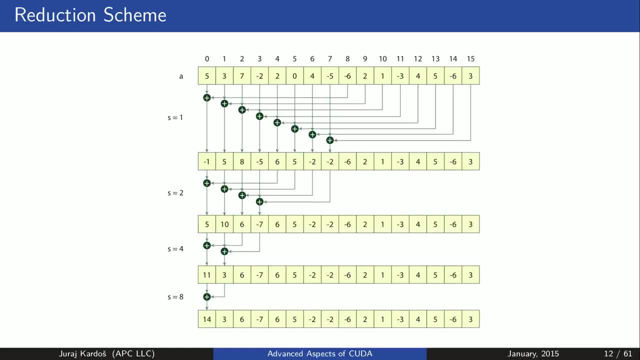 size of the array A. Each thread of this kernel computes sum of two numbers, so as a result, we have an array with half the size of input array. We continue this procedure until we have only single number left. that is the result of the reduction. 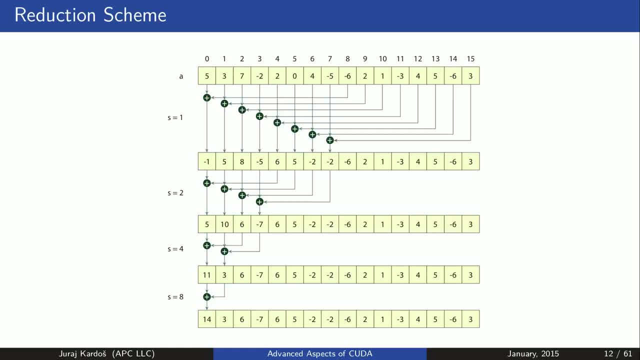 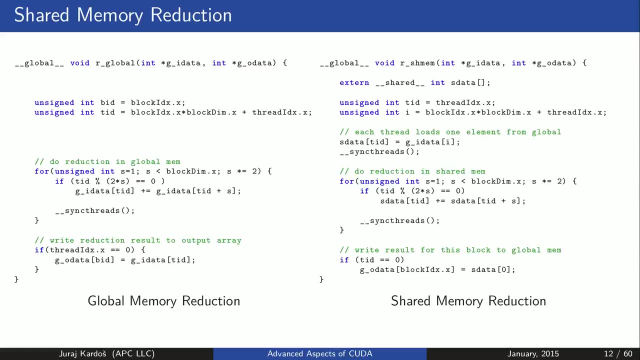 You will see this reduction performed in global memory and its modification using shared memory, so that you can see what is the impact of shared memory to the performance. In this example, we will compare performance of reduction in global memory and its modification that uses shared memory. 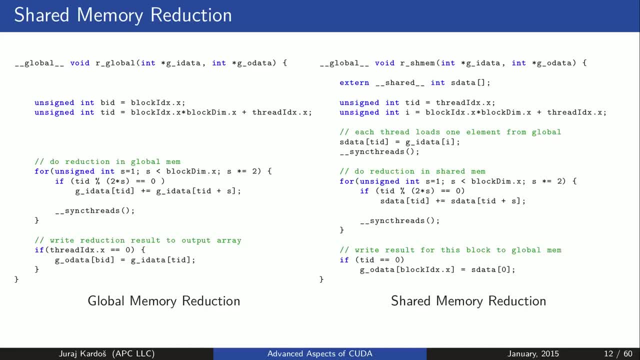 Shared memory in CUDA C device code is declared using the Shared Variable Declaration specifier. There are multiple ways to declare shared memory inside a kernel, depending on whether the amount of memory is known at compile time or not. For example, we can declare shared memory inside the kernel depending on whether the amount 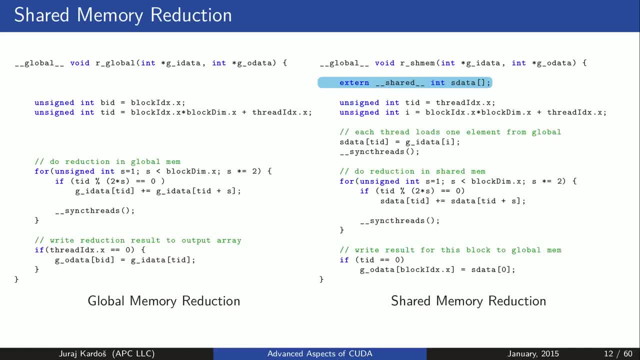 of shared memory is known at compile time or at run time. If you know amount of shared memory during compile time, you can specify the size of shared memory directly at the declaration of shared variable. In case this information is not known, we dynamically figure out amount of shared memory. 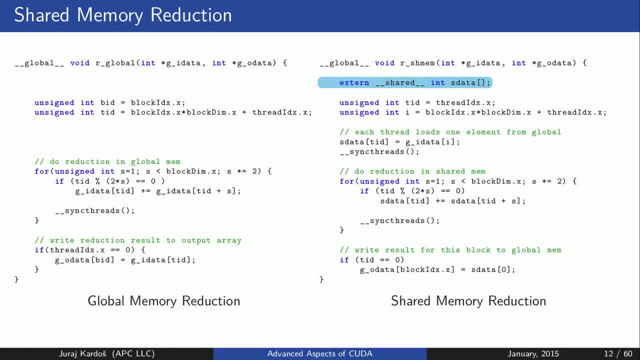 during run time and declare this information from outside kernel. therefore, keyword extern- Third argument of kernel, launch together with blocks, threads within each block is amount of shared memory. In case of shared memory reduction, we need to load data from global memory to our declared 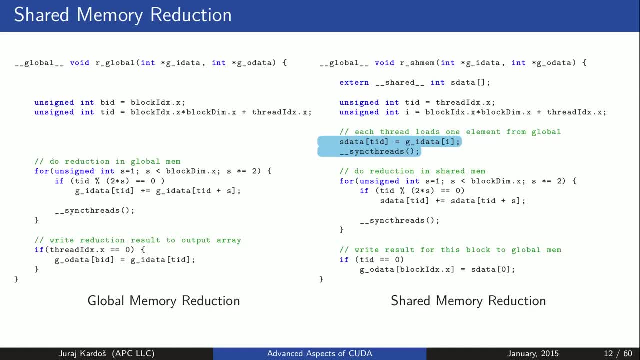 shared array. We need to synchronize threads after this operation. Let's say that two threads- thread 1 and thread 2, each load a data element from global memory and store it to shared memory. Then first thread wants to read second element from shared memory. 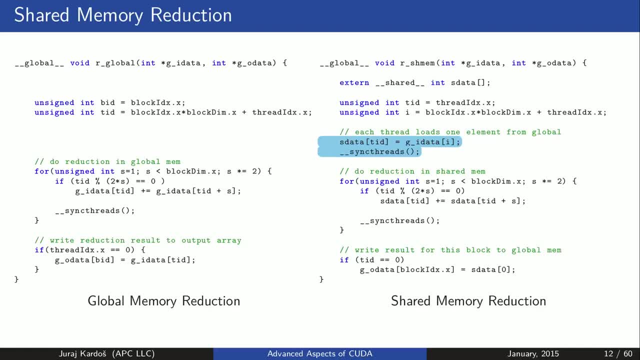 Let's assume that our two threads are shared. If second thread has not finished writing its element before the first thread tries to read it, we have a raise condition, which can lead to undefined behavior and incorrect results. Sink thread barrier ensures that threads proceed to reduction for cycle only after the shared 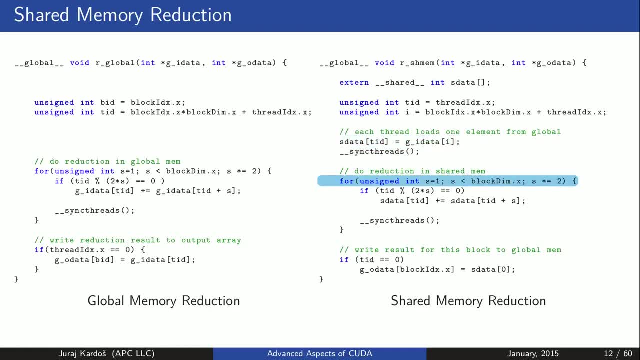 memory has been loaded from global memory. In order to efficiently use the data from shared memory, it should be reused many times. The second thread has not finished writing its element before the first thread tries to read it. we have a raise condition which can lead to undefined behavior and incorrect 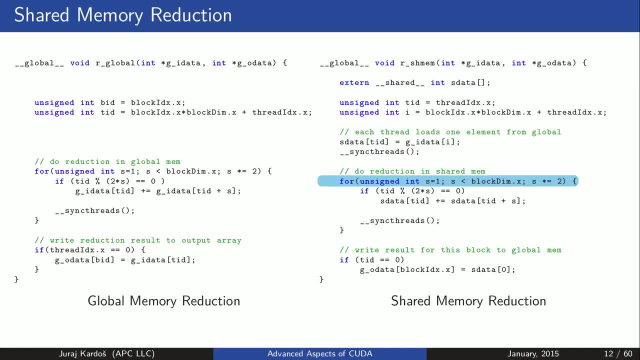 results. Otherwise there is no performance benefit, since the data first need to be loaded from slow global memory and later written back. Our application will be efficient only for big iteration variable, that is, for big thread block size, And after we finish the reduction we need to write the reduction result back to global. 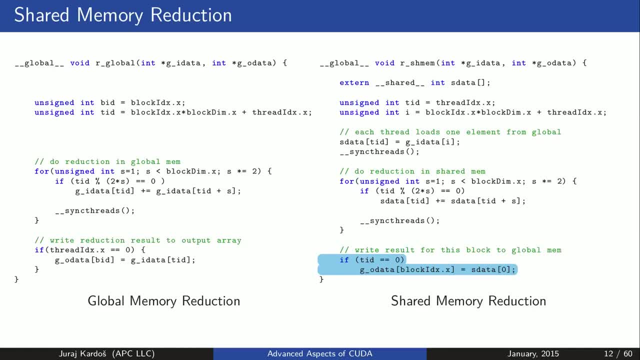 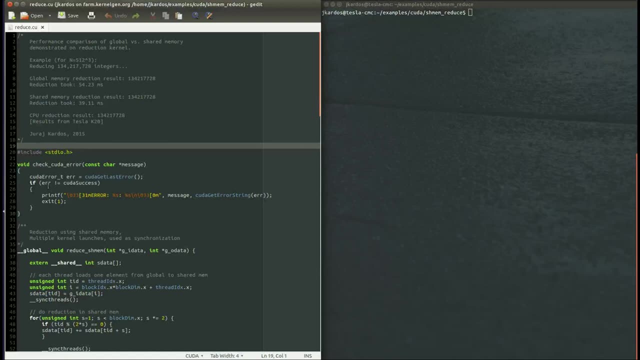 memory so that it can be further proceed in case of partial per-block results or transfered back to host after the reduction is complete. This is the demo program where we want to reduce 130 million integers. We will compare performance of reduction using global and shared memory. 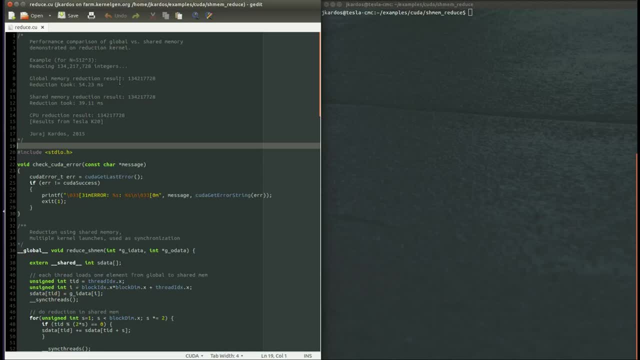 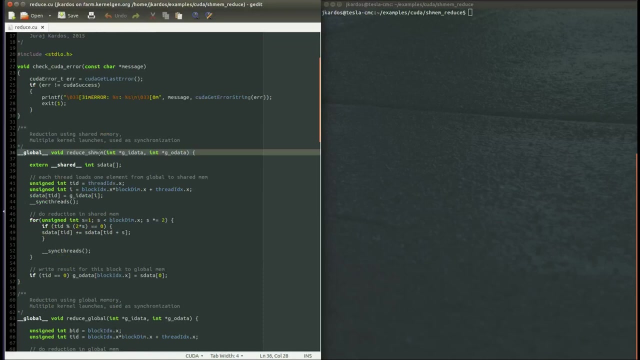 For Tesla K20, the global memory reduction took 54 ms, while the shared memory took only 49 ms. You might get different numbers depending on the used device, its architecture and some other factors. Here we have our shared memory reduction kernel. we have already seen 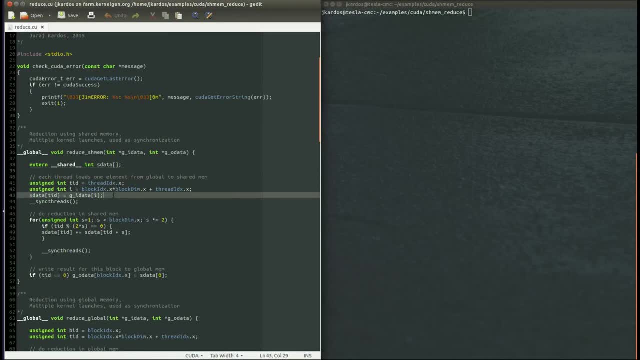 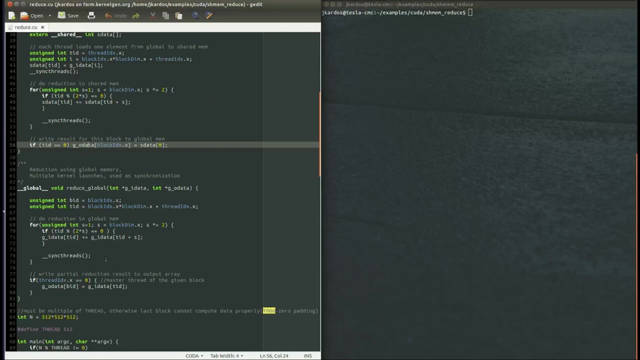 We create shared memory, initialize it by loading data from global memory and after the reduction is complete, we write the result back to global memory. Global memory reduction kernel is rather straightforward, basically the same code without the shared memory In the main function. we see standard process. 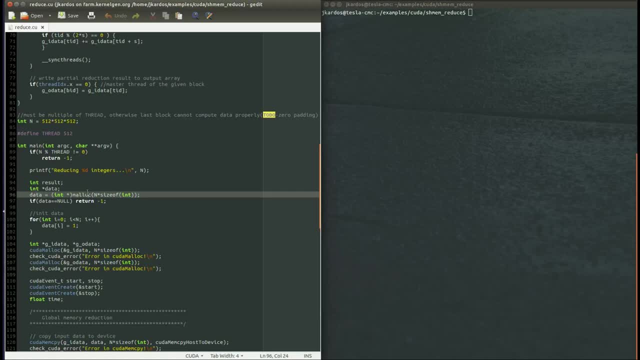 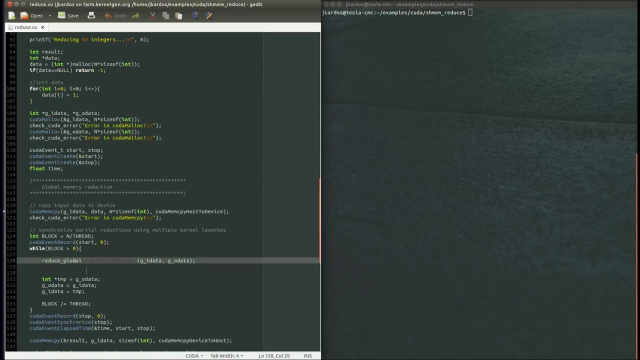 We allocate memory to hold our data. Memory is initialized to 1, so that we can easily verify the result. What is worth mentioning is that the result of calling the reduction kernel is not a single number, but rather array of partial results. 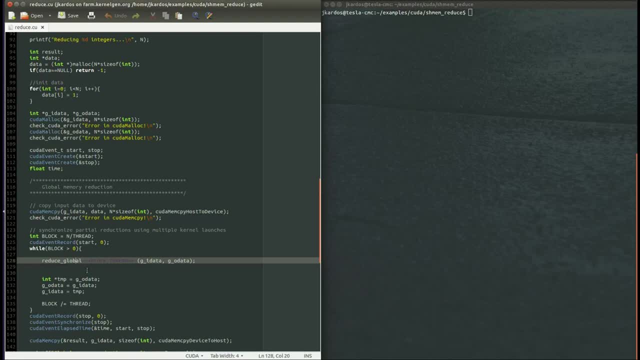 For every thread block, we get one reduction result which we need to forward the process in case we run our kernel with multiple thread blocks. So this is the result. Therefore, we repeat our kernel launch until we run it only with a single block, which 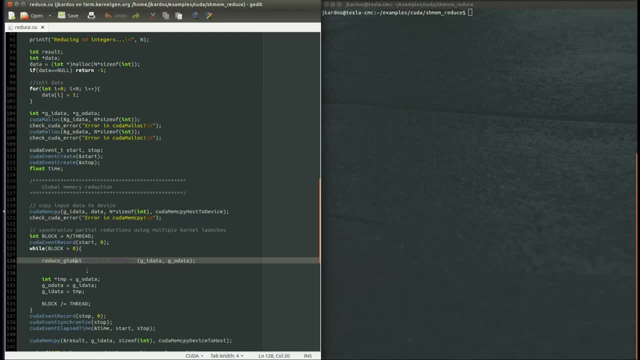 will produce the final result. The CUDA events are used to measure the elapsed time of the reduction. Basically, we mark two places in the code with CUDA event record and then compute the time difference between these places, which will get us the execution time of the given code. 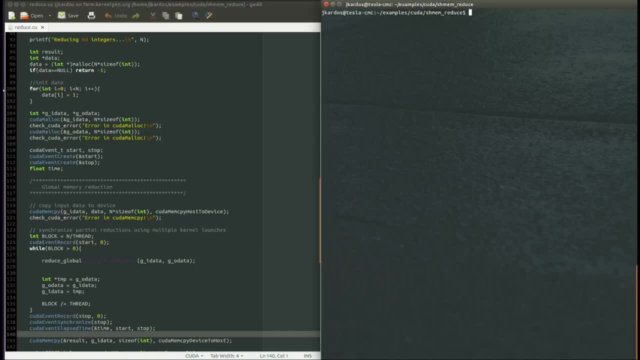 block. If we run our reduction kernel with multiple thread blocks, we will get the same result, but with multiple thread blocks. Therefore, we repeat our kernel launch until we run it only with a single block, which will produce the final result. If we run our reduction kernel with block size of 512 threads, we can compare the execution. 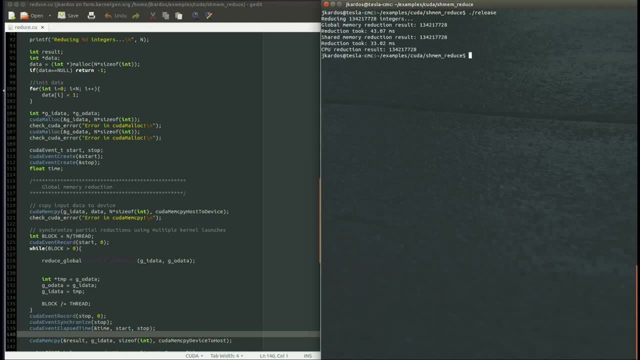 time of both kernels. We see similar numbers as we have seen before. We see some speedup, so it is really beneficial to use shared memory in case of kernels with high memory access and high data reuse ratio. In this particular reduction, there could be done more optimizations, such as coalescing. 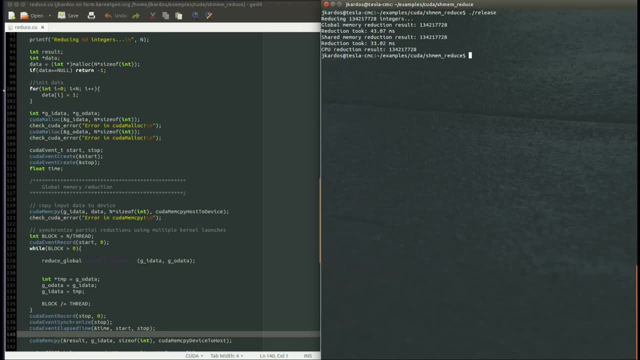 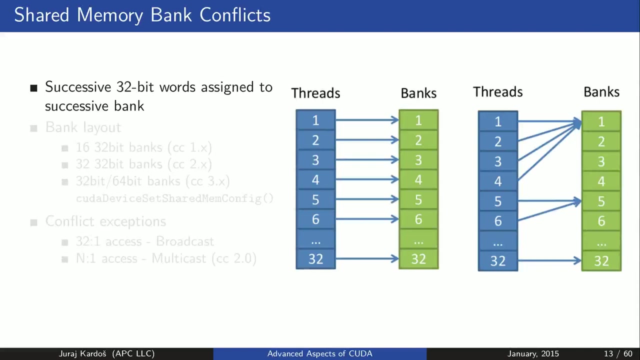 memory, removing divergent branch, etc. However, even with this simple optimization of memory access pattern, we see some speedup To achieve high memory bandwidth for concurrent accesses. shared memory is divided into equally sized memory modules that can be accessed simultaneously. 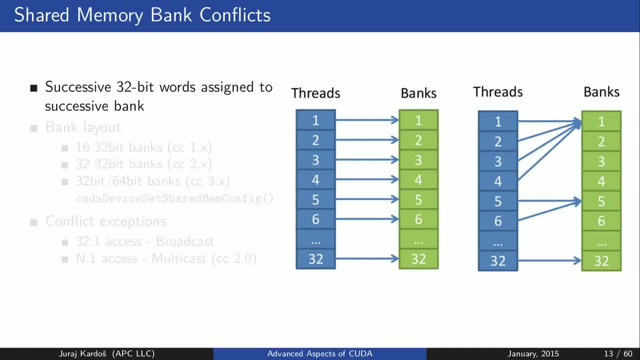 However, if multiple threads requested addresses map to the same memory bank, the accesses are serialized. The hardware splits a conflicting memory request into as many separate conflict-free requests as necessary, decreasing the effective bandwidth by a factor equal to the number of colliding memory requests. 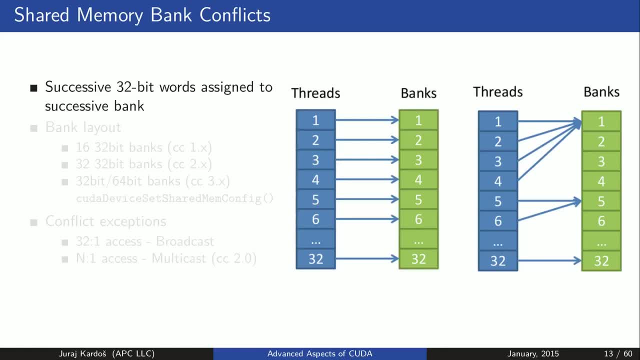 Shared memory banks are organized such that successive 32-bit words are assigned to successive banks. Each bank can service one address per cycle, So that shared memory can service multiple addresses per cycle. So that shared memory can service multiple addresses per cycle. So that shared memory can service as many simultaneous accesses as it has banks. 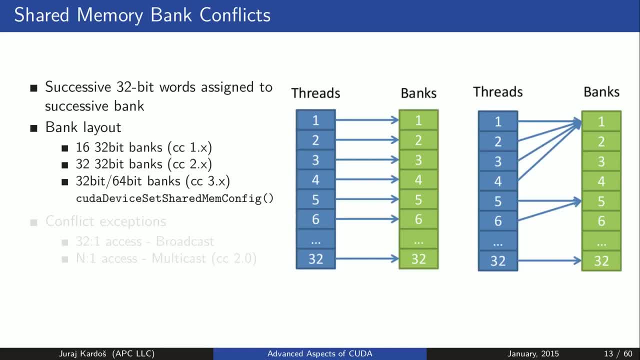 For devices of compute capability 1,. the warp size is 32 threads and the number of banks is 16.. A shared memory request for a warp is split into two requests. For devices of compute capability 2,, the warp size is 32 threads and the number of banks. 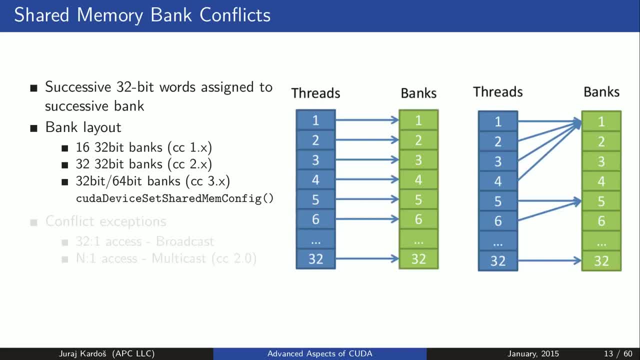 is also 42. Therefore, a whole warp can be serviced in one request. Devices of compute capability 3 have configurable bank size, which can be set to either 4 or 8 bytes. Setting the bank size to 8 bytes can help to avoid shared memory bank conflicts when 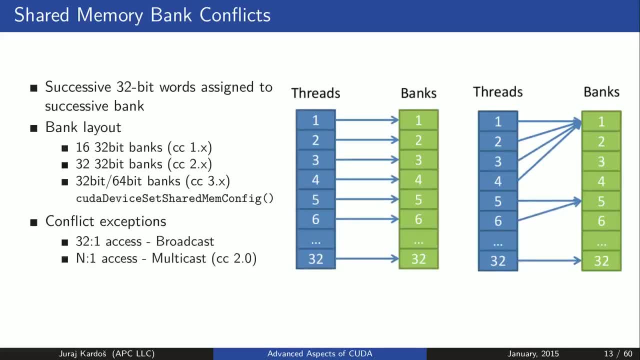 accessing double precision data. In the left use case scenario, different threads are accessing different banks. therefore there are no conflicts. In the other use case, first four threads are accessing the same memory bank, which will result into conflict and serializing requests into four consecutive memory accesses. 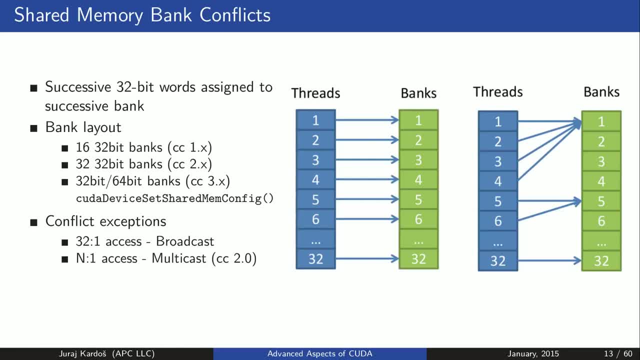 Exception to the bank conflict is broadcast when all threads from warp request read operation from the same bank, resulting into memory broadcast. Another exception is when multiple threads request the read from the same memory bank, which will result into multicast. This optimization is very simple. 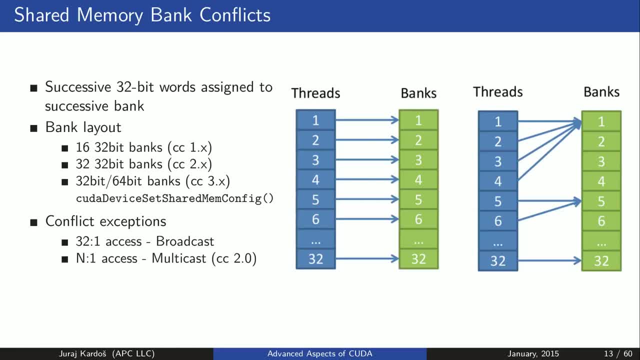 This optimization was introduced in Fermi architecture. This concludes our part on shared memory. Next part, we will have a look on efficient data transfers. 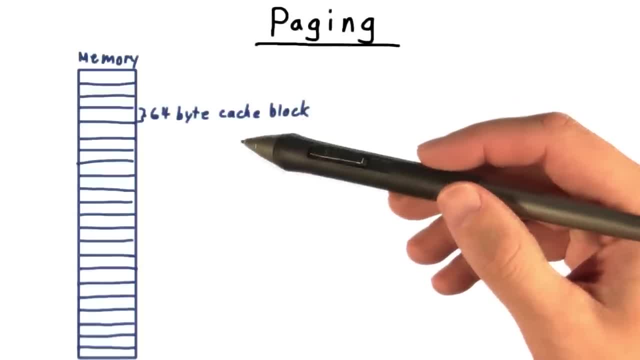 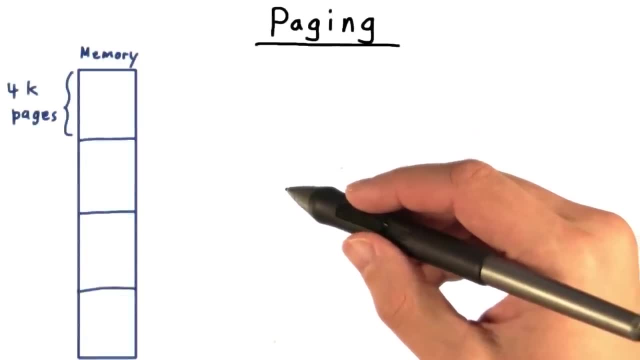 Recall how, for caches, we divided memory into blocks or cache lines, and this is the granularity at which caching operates. Similarly, for a paging system, we divide up our physical address into pages, often 4K long. Pages are the granularity at which we grant memory to processes. 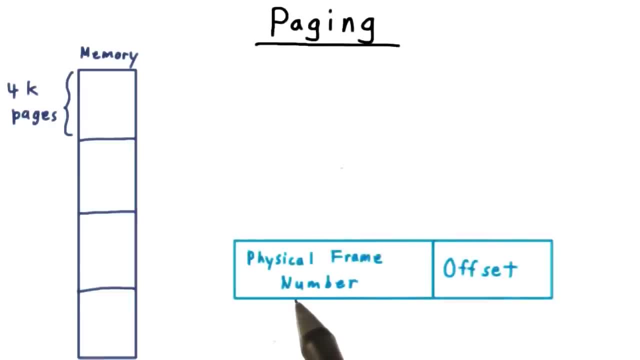 The higher order bits determine the page number, also called the physical page frame, and the lower order bits determine the offset into the page Correspondingly, the virtual address space is similarly divided into pages. Again, lower order bits determine the offset within a page. 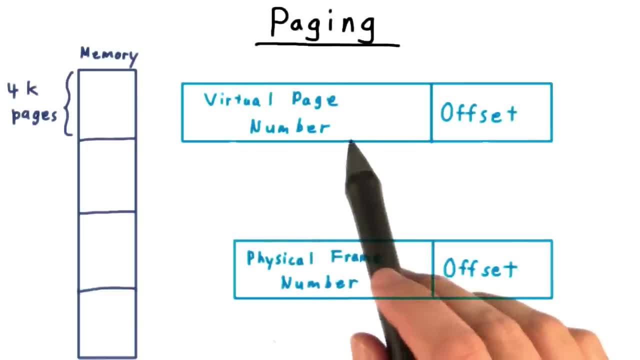 The higher ones determine the virtual page number. The number of bits in the offset always matches. That's because virtual page sizes and physical page sizes are necessarily the same. But the number of bits involved in the virtual page number need not match the number of bits used to identify the physical frame number. 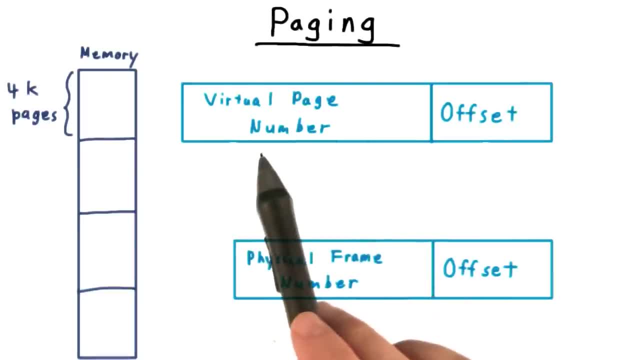 That's because, as we've said before, it's possible to have more virtual pages than physical pages. Since we are mapping page for page between virtual and physical addresses, the offsets stay the same. We do need to translate page numbers, however.